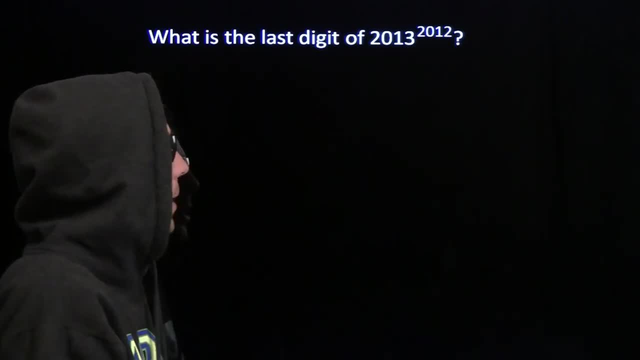 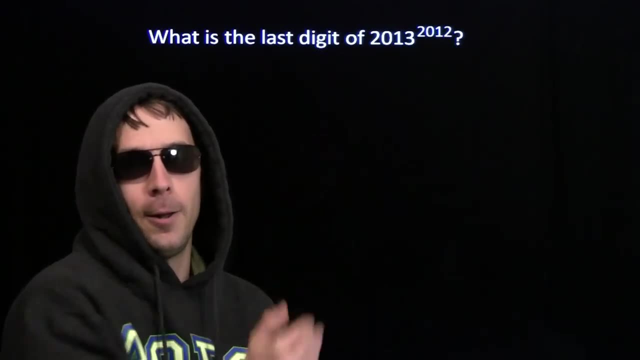 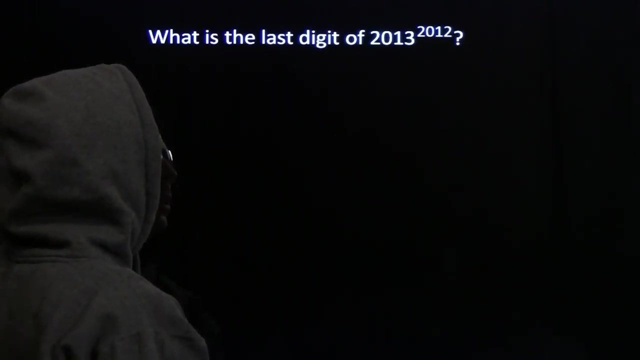 here We're looking for the last digit of 2013 to the 2012.. I got nothing smart. so what's the stupid thing to do? Stupid thing to do is just multiply it all out. It's not just stupid, it's completely crazy. But ugh, got nothing else. Well, we'll get. 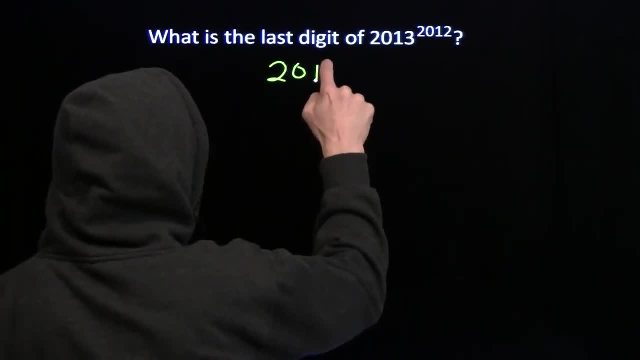 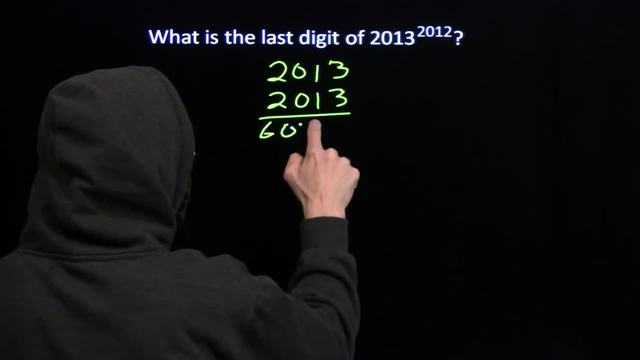 started just by multiplying out 2013 squared. Multiply that by itself, Let's see I'm up- by 3 times the 2013.. You get 6039.. And the 1 here the 10, we're going to multiply. 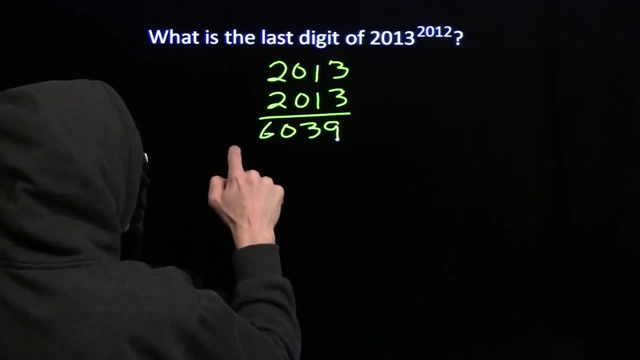 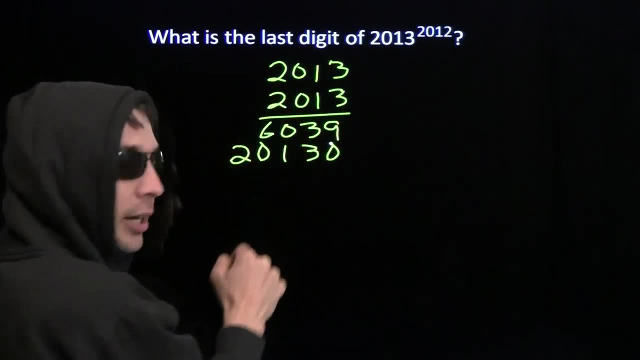 this 2013 by the 10 from the 1 there in the tens place and we'll get 20130. And the zero is not going to give us anything interesting. Then we're going to multiply by 2000 for the 2 out here in the thousands place and we've got our three trailing zeros there. And then 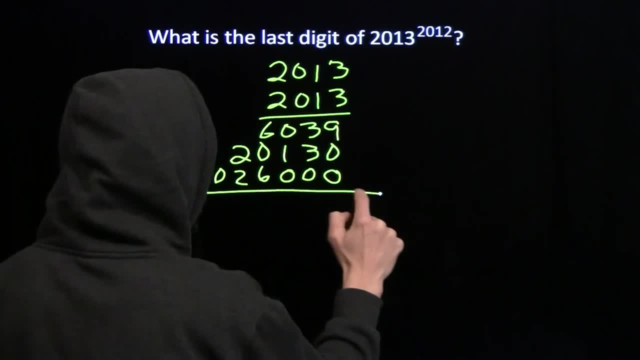 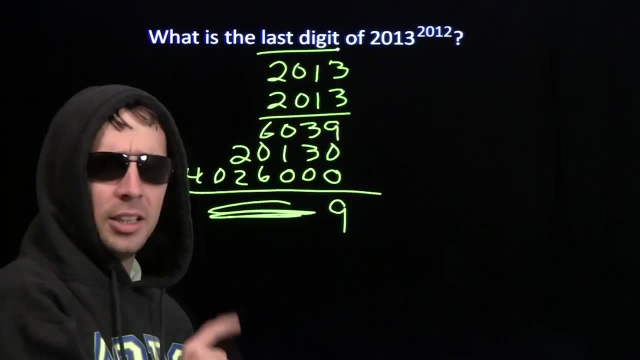 we've got 4026.. Then we add that all up and we get the 9.. And then actually we don't care about any of this stuff out here. All we care about is the last digit And check this out. All we care about is the last. 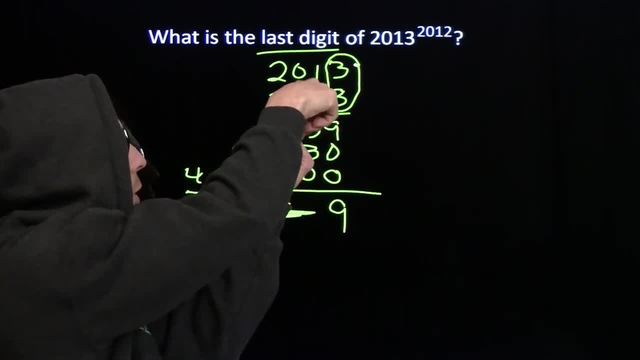 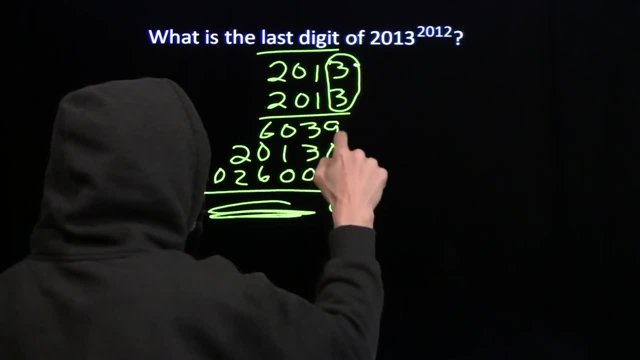 digit. We get the last digit just from multiplying the last digits of the two numbers that we started with. We don't even care about the rest of the numbers. The 3 times the 3 is going to give us the last digit here. It's going to give us the 9.. All this other stuff. 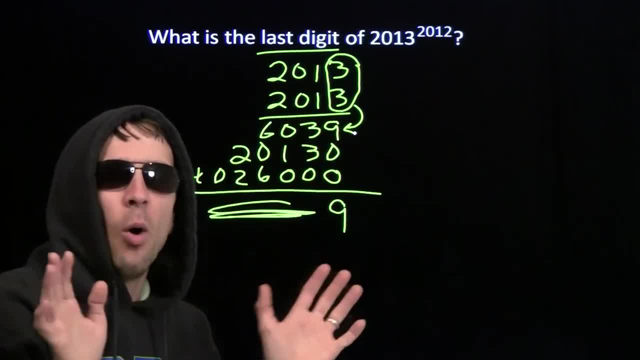 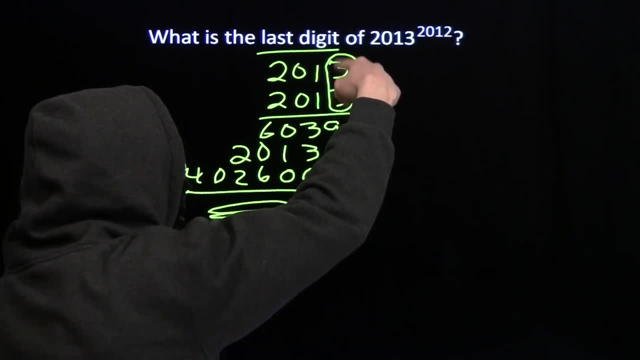 is just going to affect the tens, the hundreds, the thousands and all those other digits that we don't care about. Whenever you multiply two numbers to get the digit of the product, all you care about is the product of the last digits of the original. 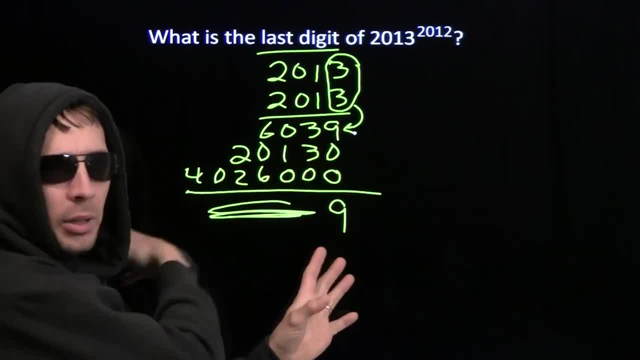 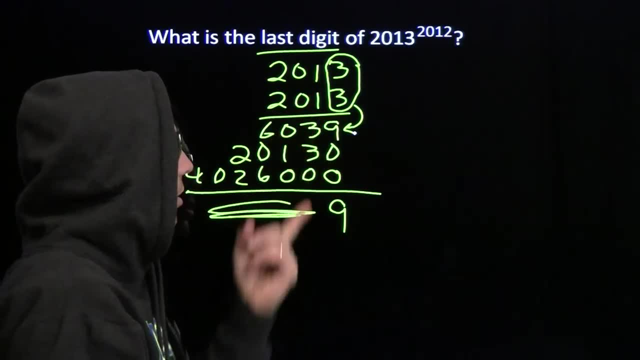 numbers, All these other numbers are just going to affect higher places in the number: the tens, the hundreds, all that other stuff we just don't care about. So all we need to look at are the last digits of the numbers we're multiplying. 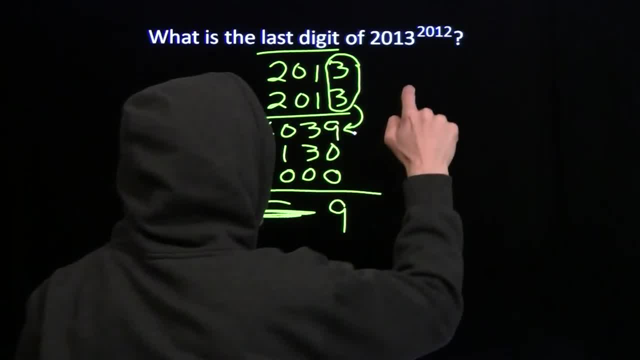 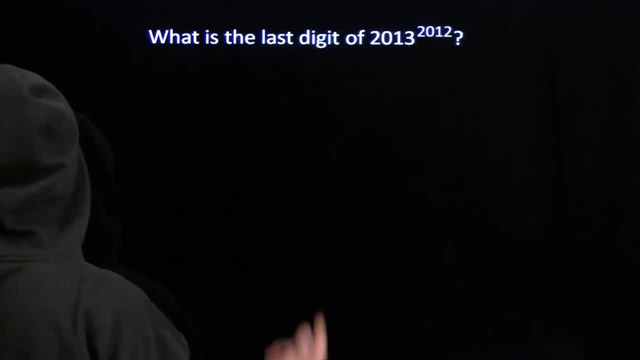 So when we're looking for the last digit of 2013 to the 2012,, all we're really looking for is the last digit of 3 to the 2012.. In other words, when you start off looking at a problem like this, you're really looking. 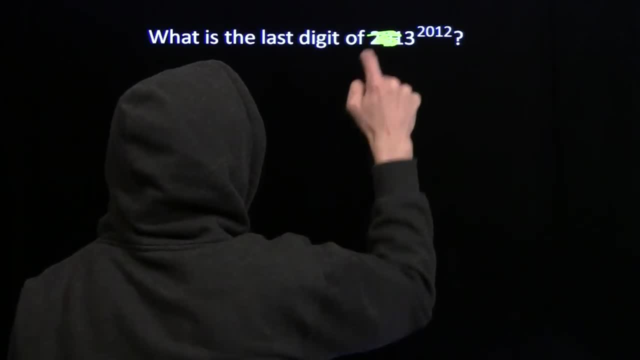 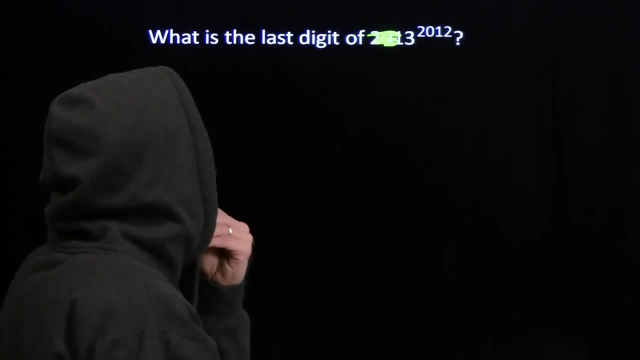 at a problem like this, And now I still don't know what to do. 3 to the 2012,. I mean, that's not as bad as multiplying out 2013 to the 2012,, but that's still going to take forever. 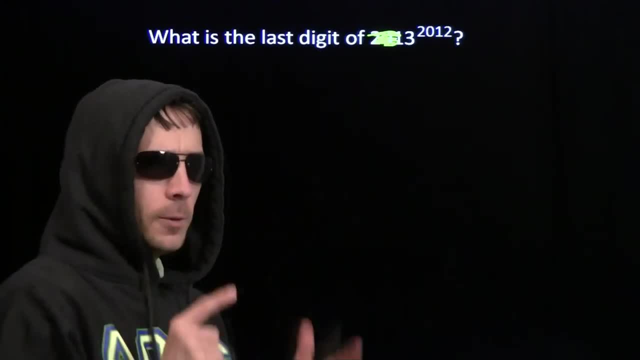 But I've got nothing better, so do something stupid. Let's start pounding out some powers of 3.. But I'm not going to do that, But all we care about is the last digit. so we're just going to look at the last digits. 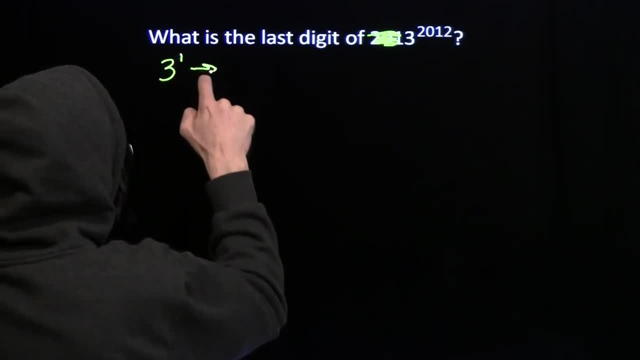 of these powers. So we'll start off with 3 to the first is easy, 3 to the first, that's just 3.. Then 3 squared. we get to 3 squared by multiplying the 3 by 3, that's going to end in 9.. 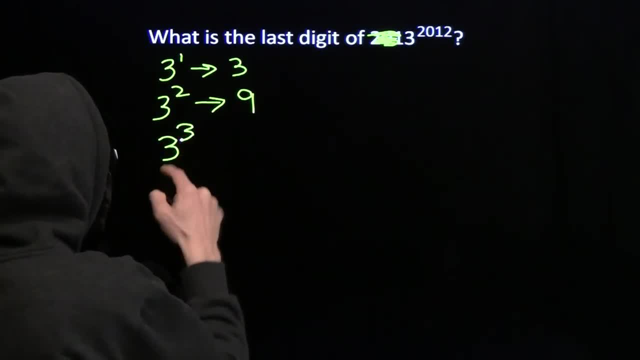 That's even going to be 9.. Three cubed. well, we'll get to 3 cubed by multiplying the 3 squared by 3.. Multiply 9 by 3, you get something that ends in that's right 7.. 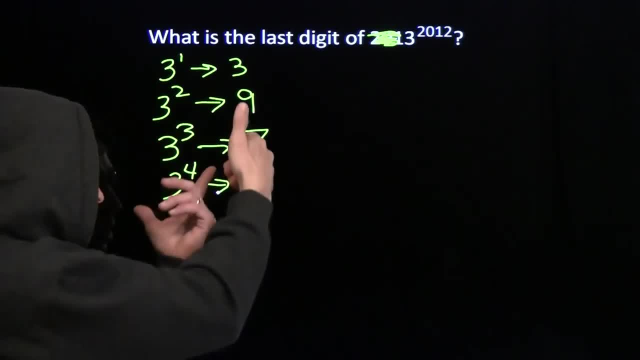 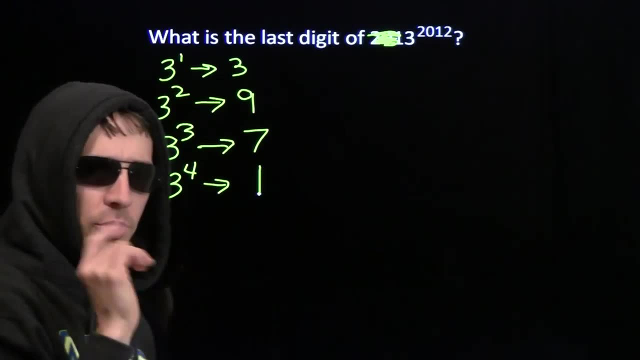 Three to the fourth, three to the fourth. multiply the 3 cubed by 3, means you're multiplying something that ends in 7 by 3, you're going to get something that ends in 1.. All right, 4 down, 2008 to go. 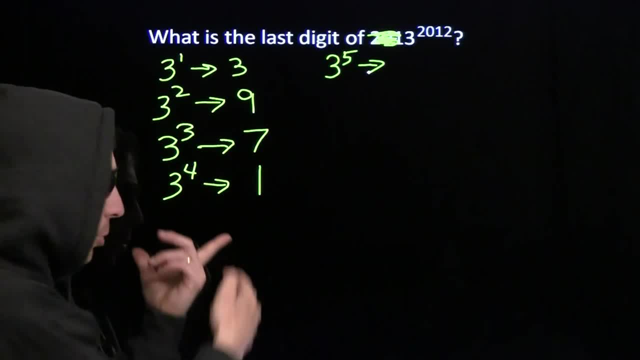 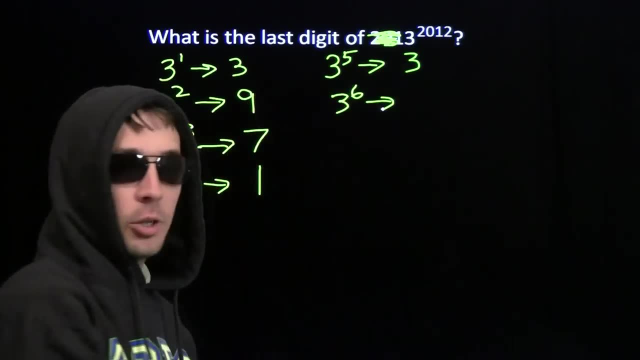 Three to the fifth: we're going to multiply this 3 to the fourth by 3, multiply 1 by 3, you get 3.. Three to the sixth: we're going to multiply 3 to the fifth by 3, 3 to the fifth ends in. 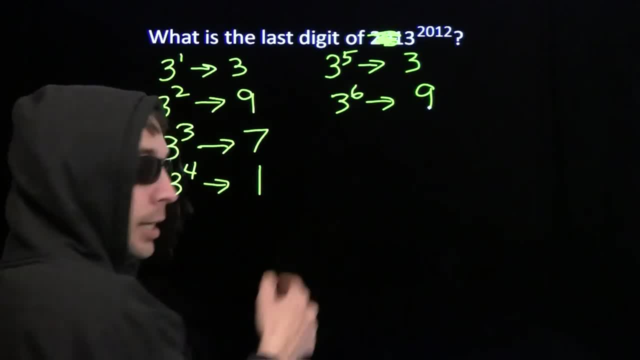 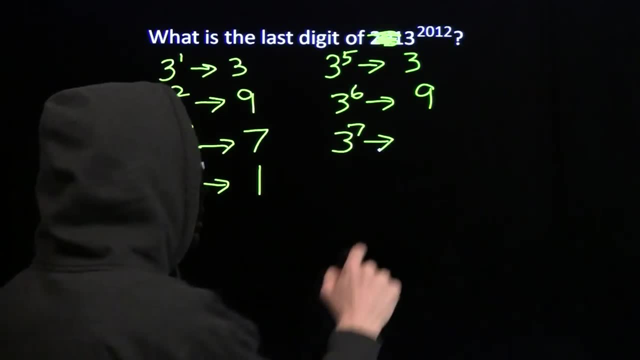 3, multiply that by 3, you get something that ends in 9.. Now we're going to multiply by another 3, that'll give us 3 to the seventh. Multiply something that ends in 9 by 3.. You get something that ends in 7,, just like we did over here. 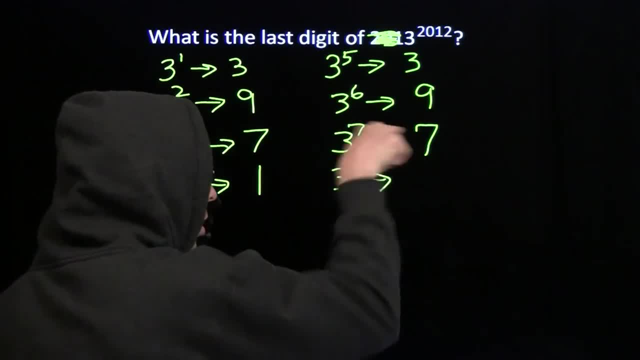 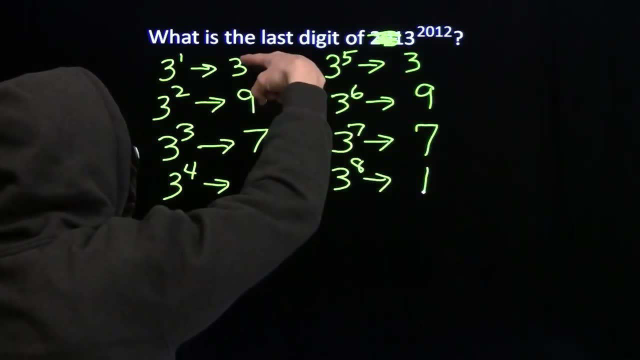 Three to the eighth. multiply 3 to the seventh by 3,, you get 3 to the eighth. Multiply something that ends in 7 by 3,, you get 1.. We did the same thing over here that we did here, and we can even see why. 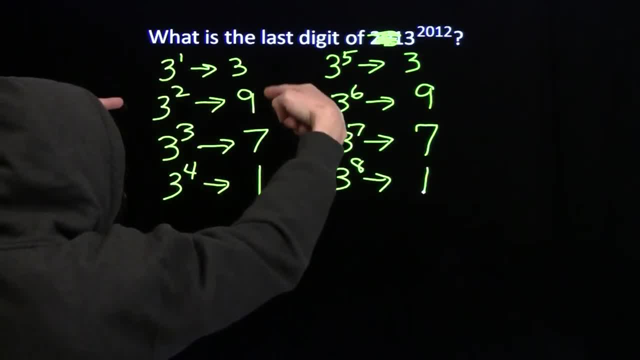 Once we have this 3 again, we're going to get to the next row just by multiplying by 3.. That's the same thing we did over here: Going to get to the next row, going from 3 to the sixth to the seventh by multiplying. 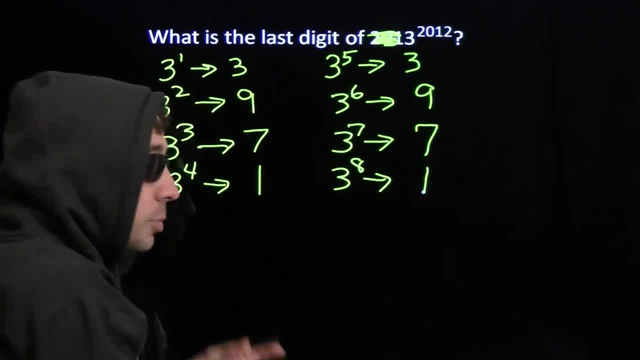 by 3, just like we did over here: 3 to the seventh to 3 to the eighth. we're just multiplying by 3, just like we did over here. We're just repeating the same four steps and this next one: multiply by 3, you get. 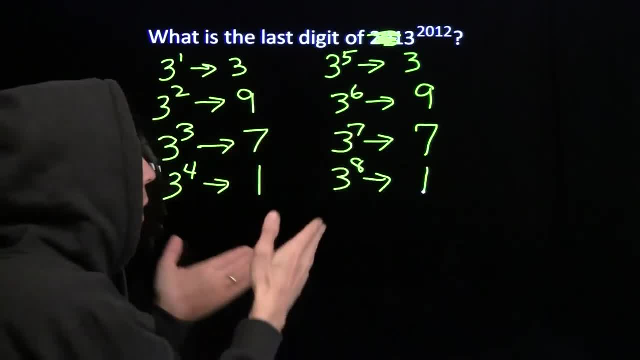 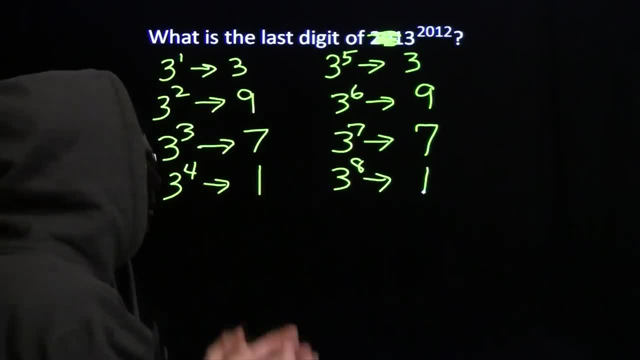 3 to the ninth is going to end in 3.. And around we go. We found a pattern. And how did we find that pattern? We did something stupid and something good happened. We see this pattern now that the last digits of the powers of 3, they go in these cycles. 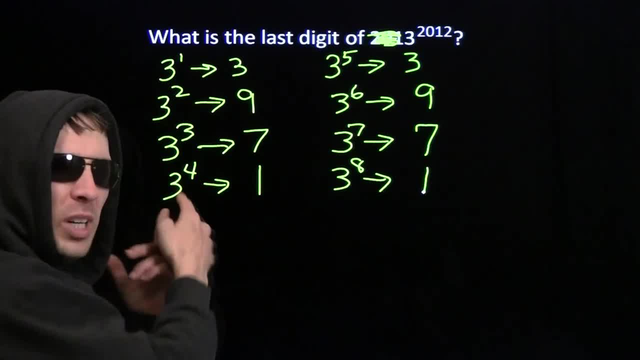 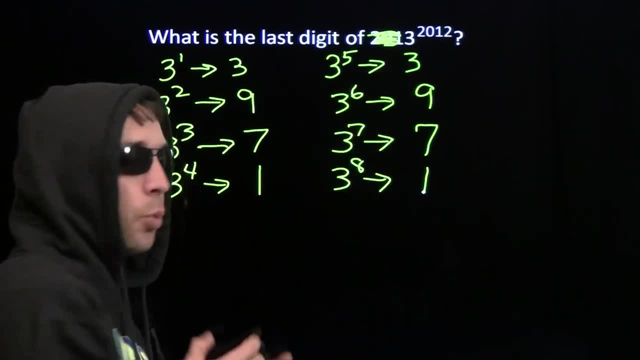 of 4, 3, 9, 7, 1, 3, 9, 7, 1, so you raise 3 to any multiple of 4,, you get a number that ends in 1,. 3 to the 2012th, 2012 is a multiple of 4, so we know that the last digit of 3 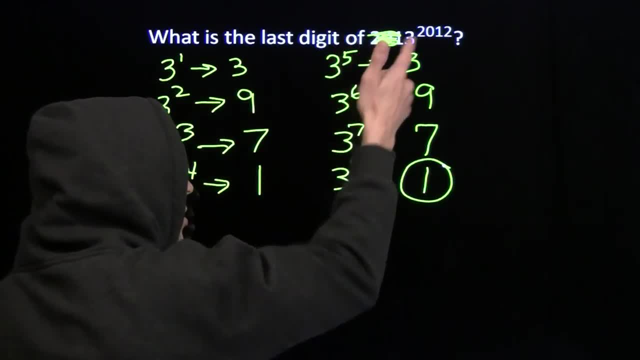 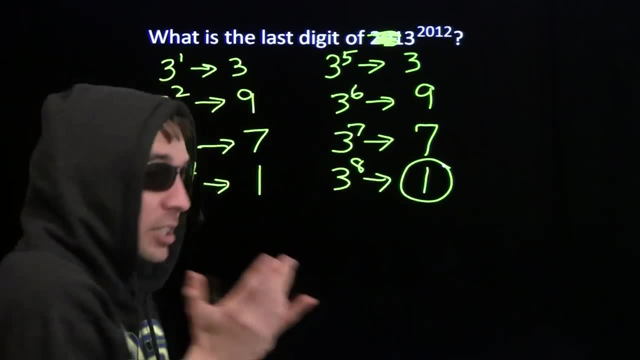 to the 2012th is 1, so that means the last digit of 2013 to the 2012th is 1.. So we used our key strategy there- do something stupid. and we discovered another great strategy, which is find a pattern. 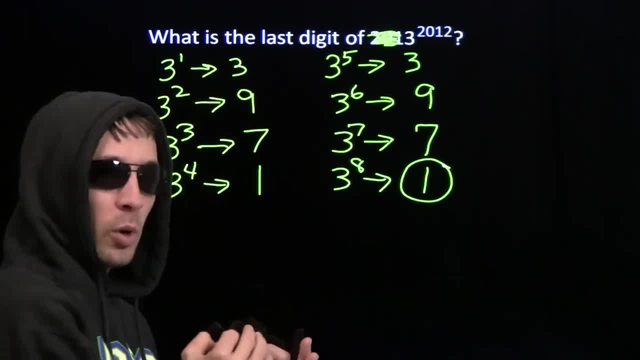 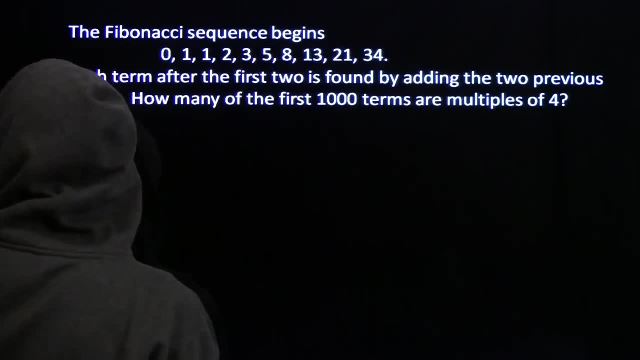 Now it wasn't enough just to find a pattern. we had to make sure that the pattern really worked. We figured out why the pattern was true. Now Let's look at these two strategies on this problem right here. Here we've got a sequence. it's called the Fibonacci sequence, and here's how it works. 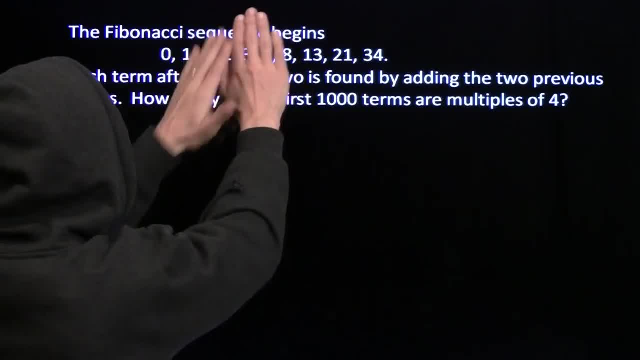 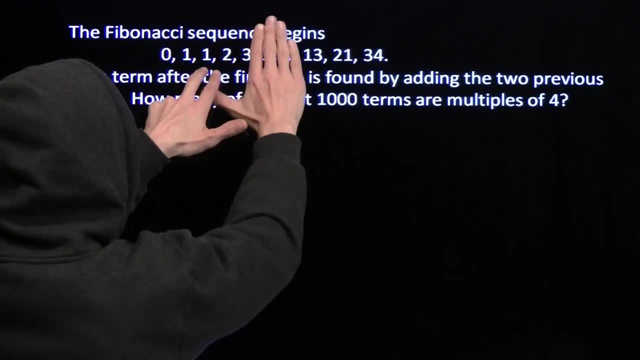 We start off with 0, 1, then each term after that you get by adding the two terms before it: 0 plus 1 is 1,, 1 plus 1 is 2,, 1 plus 2 is 3,, 2 plus 3 is 5,, 3 plus 5 is 8, you get the. 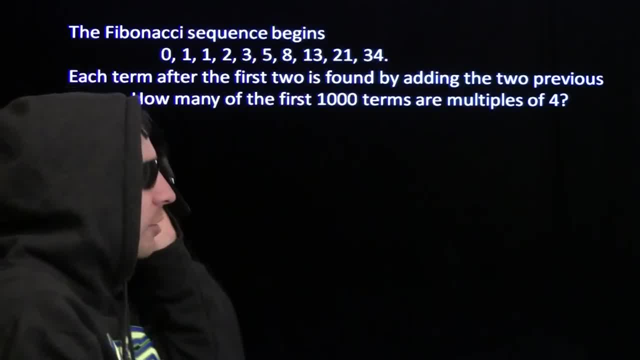 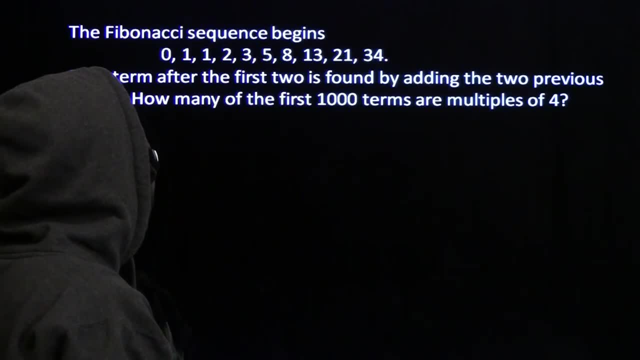 picture. Now we want to find out how many of the first thousand terms, if we just keep going with this, are multiples of 4.. Yeah, I don't see it. I don't see the answer right away, so here we go. 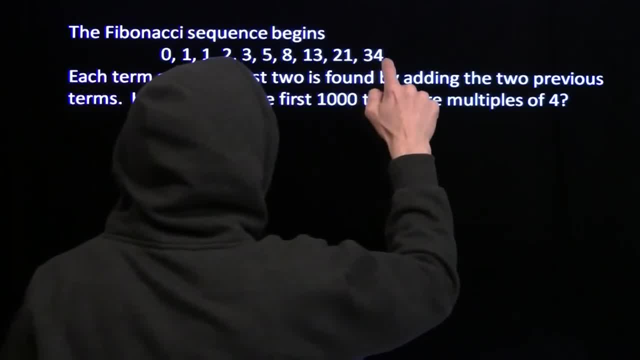 Can't do something smart, do something stupid. Let's just keep listing some more terms. I got one multiple of 4 right there. I got another multiple of 4 right there. Let's see if we can find some more. 21 plus 34 is 55.. 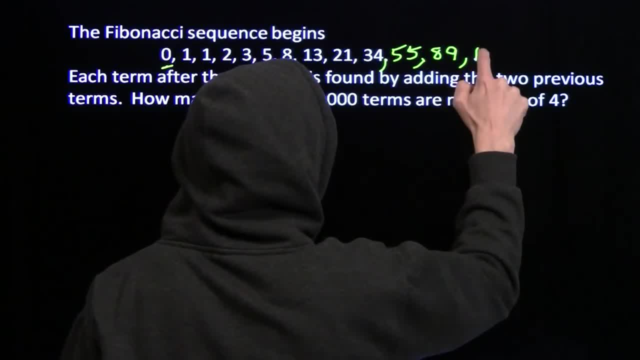 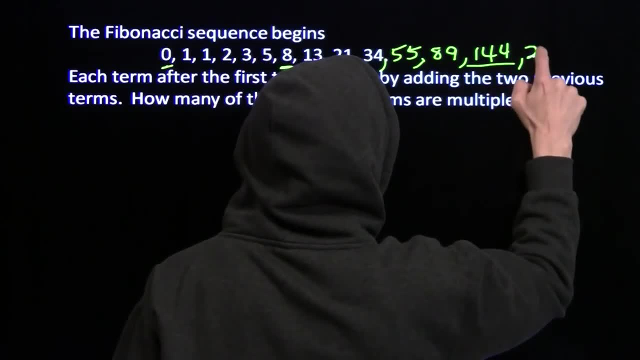 34 plus 55 is 89.. 55 plus 89 is 144.. We have a winner. There's another multiple of 4.. 89 plus 20.. plus 144 gives us 233.. I don't want to keep doing this, but check this out. There's one. 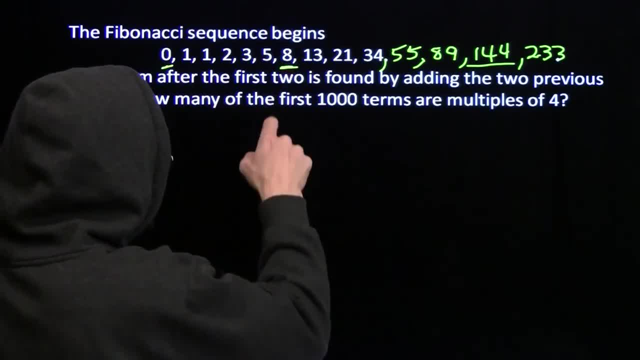 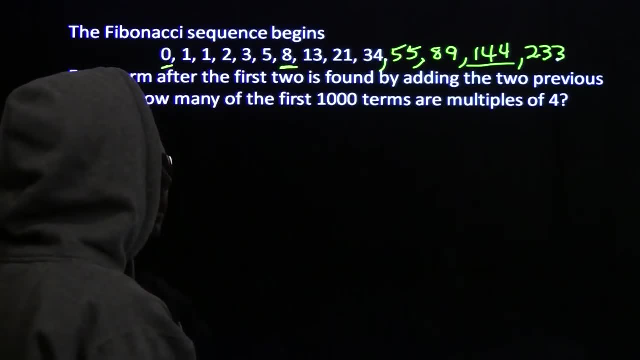 here, then I skip five terms and get to another one. then I skip five terms and get to another one. Is that going to keep happening? It would be nice if that were the pattern. but how do I think about whether or not a number is a multiple of four? Well, I divide four into. 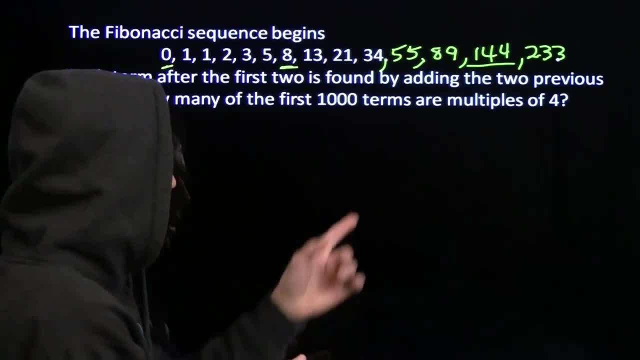 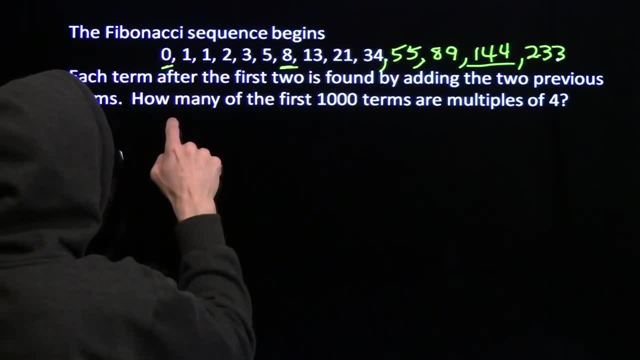 it, and if the remainder is zero, I've got a multiple of four. If the remainder is anything else, I don't. but let's just look at those remainders. We don't actually care what the numbers are. Let's take a look at what those remainders are. So the first term when I 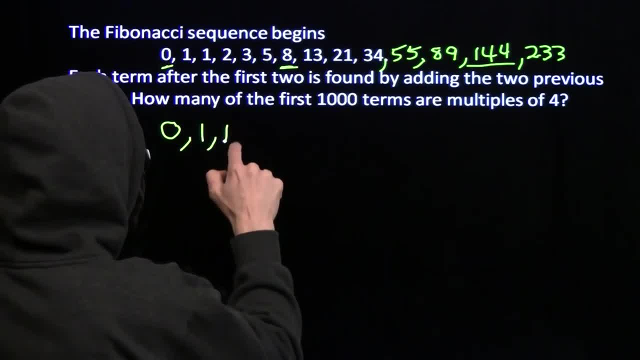 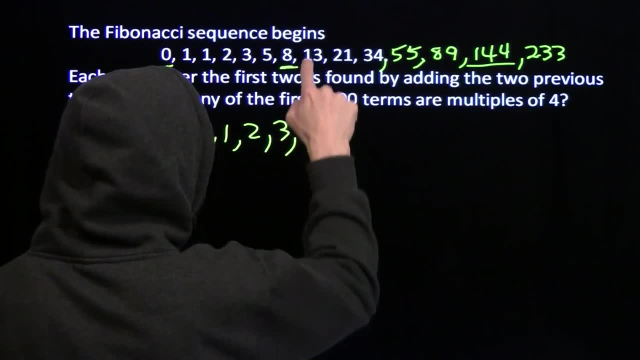 divide it by four, the remainder is zero. That's pretty easy, and the next few terms are really easy as well: Two, three and five. When I divide five by four, I get a remainder of one, and then eight gives me zero, Thirteen gives me one. Wait a second. Twenty-one that'll. 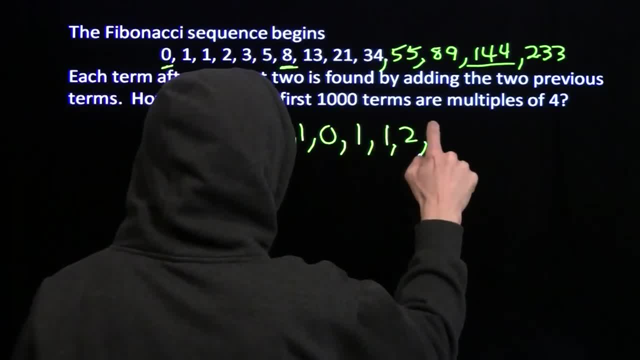 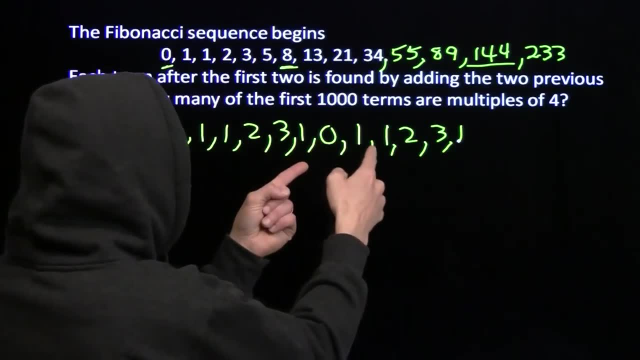 give me one, Thirty-four gives me two, then three, then one. Do you see it repeating? I see a pattern: zero, one, one, two, three. one zero one one, two, three, one, And the next one, sure enough, is zero, and then one, and then dot. 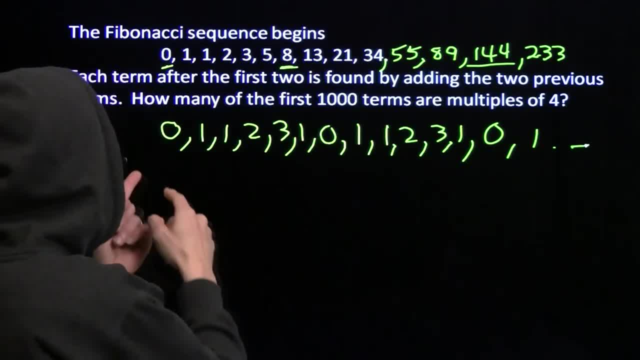 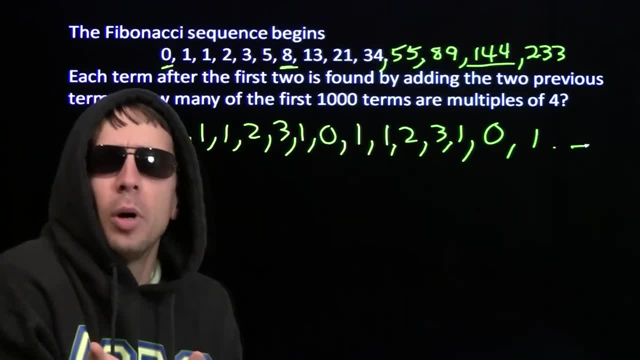 dot and then so on. What's going on here? Well, if I take a number that's a multiple of four and I add a number that's one more than a multiple of four, well that sum is going to be one more than a multiple of four. So that's why the remainder of the next term 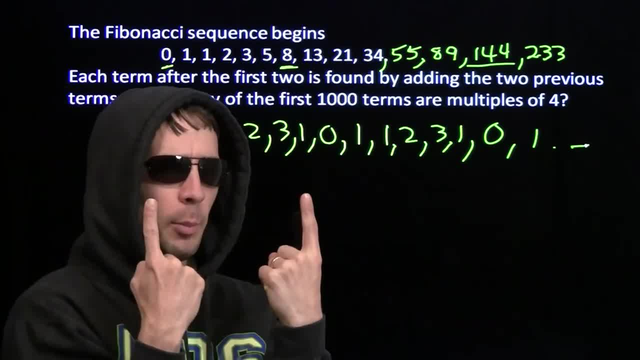 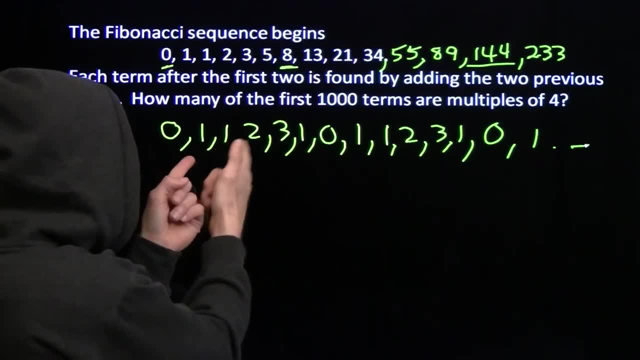 is going to be one If I take two numbers and both of them leave a remainder of one. when I divide by four and I add those two numbers together, well, those two- one, two and ones that are left over- are going to combine and become a two. One plus one is 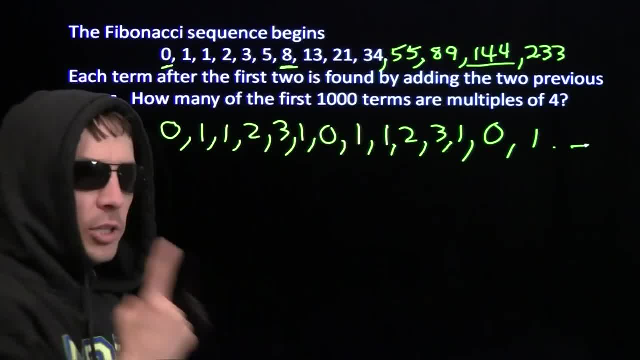 two- Yeah, I bet you knew that. one. One plus two. if I take a number that's one more than a multiple of four and add a number that's two more than a multiple of four, those left over are going to combine. We're going to have a number that's three more than a multiple. 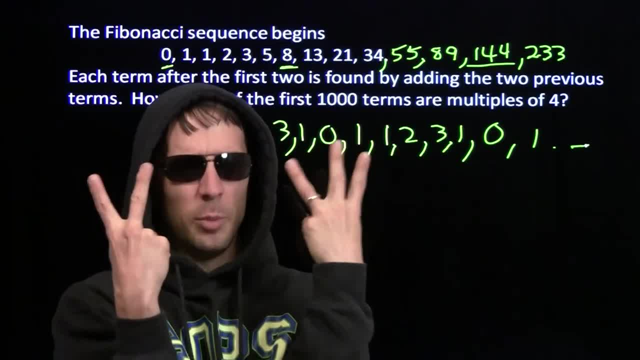 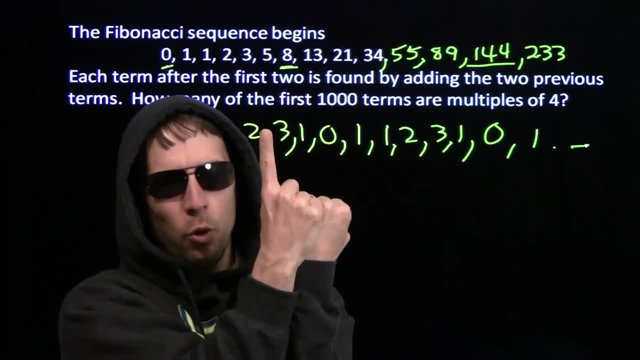 of four. If I take a number that's two more than a multiple of four and add it to a number that's three more than a multiple of four, they're going to combine. but I've got a whole four there. I can knock out a four. I've got a number left that's one more than a multiple. 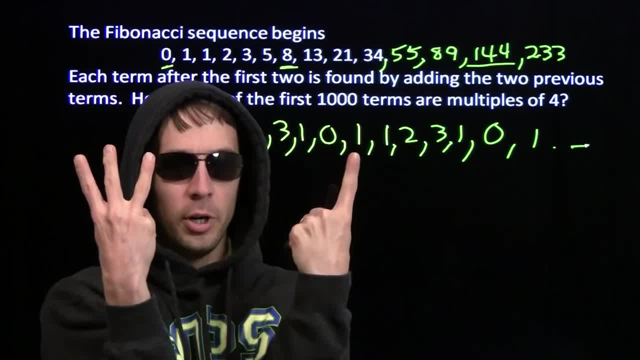 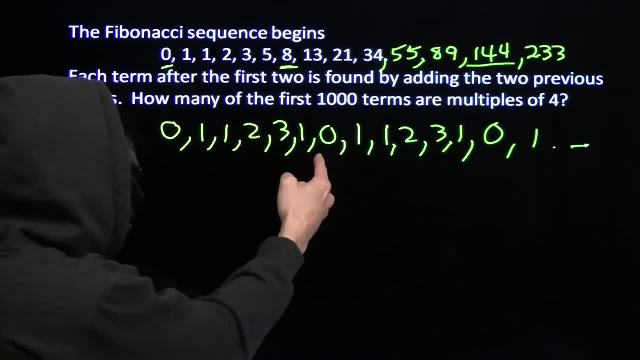 of four. Then if I take a number that's three more than a multiple of four and add it to add to a number that's one more than a multiple of four, I get a number that's four more than a multiple of four. that means I get another multiple of four. the remainder is going to: 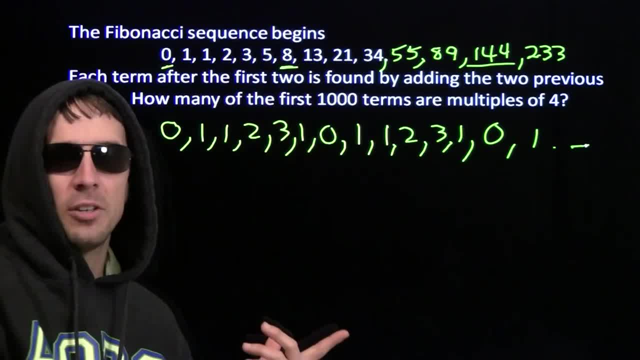 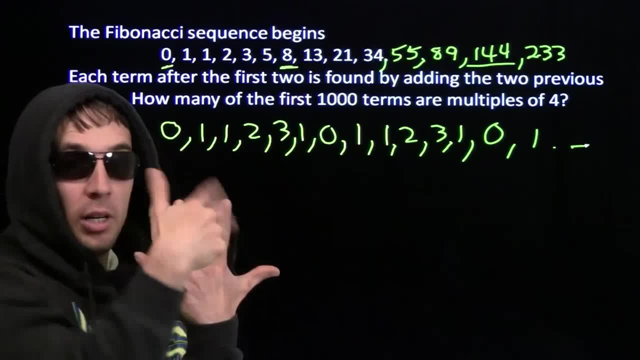 be zero. These remainders kind of follow the same relationship as the Fibonacci sequence: zero and one is one, one and one is two, one and two is three, two and three is five. but that means the remainder, when I divide by four, is going to be one, three and one is zero. one and zero. 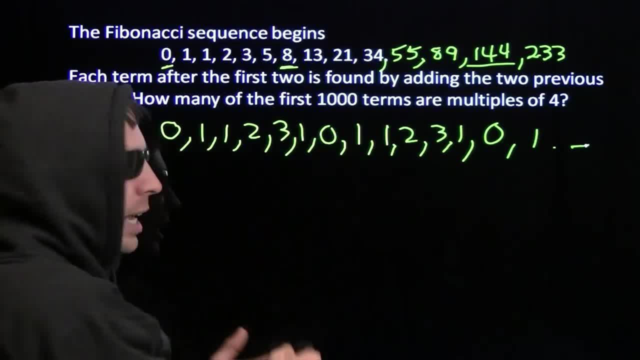 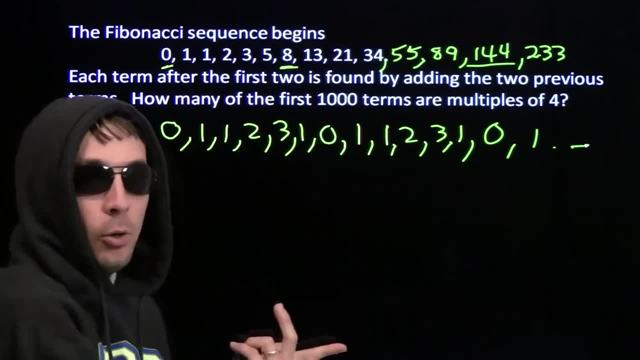 is one. And now we're back to the same starting point, And since we generate each term in this sequence just by combining the two before it, one and one. once I repeat two terms, I know the whole thing's going to repeat. 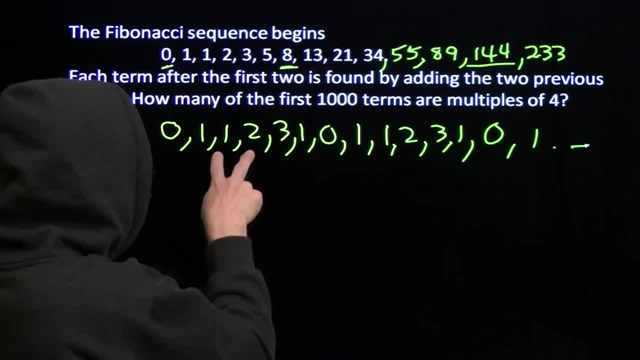 I combine the zero and one to get this one. I combine this one and one to get that two. I combine this one and two to get that three, and so on. So once I have a zero one here and I see another zero one here, I know that everything. 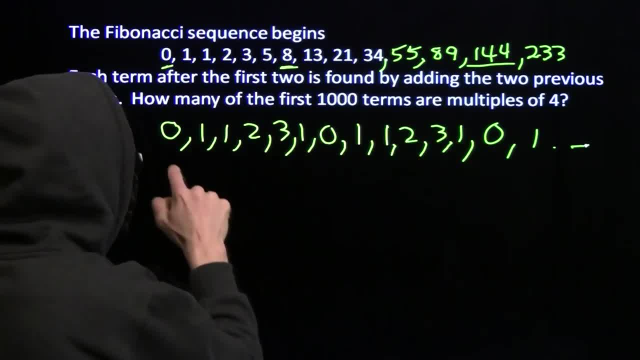 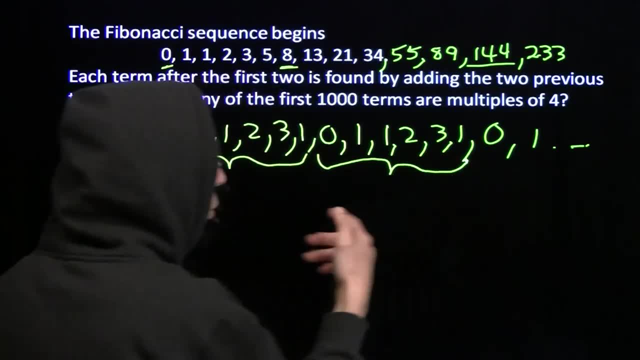 that's going to happen after this is going to be the same as what happened after this. This whole block is going to repeat over and over and over These little blocks of six. we've found a pattern and we've explained why it's there. 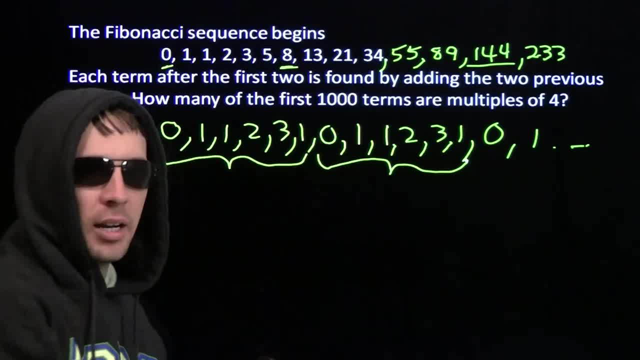 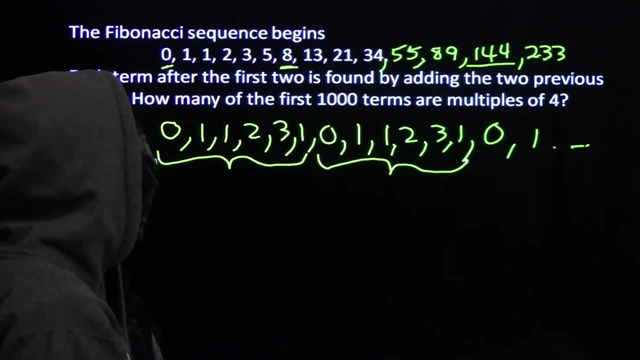 We know that these terms are going to come in blocks of six like this, and in each block of six we're going to have one multiple of four. So now I just have to figure out how many blocks of six are in this thousand. 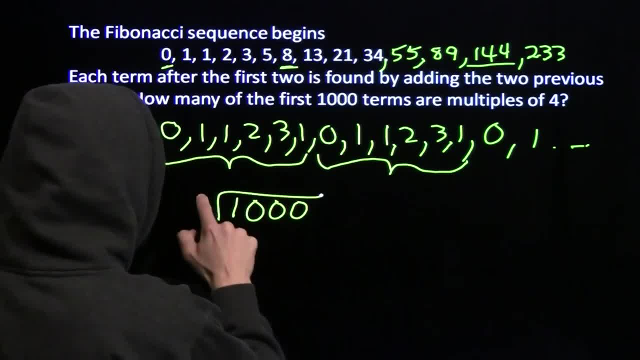 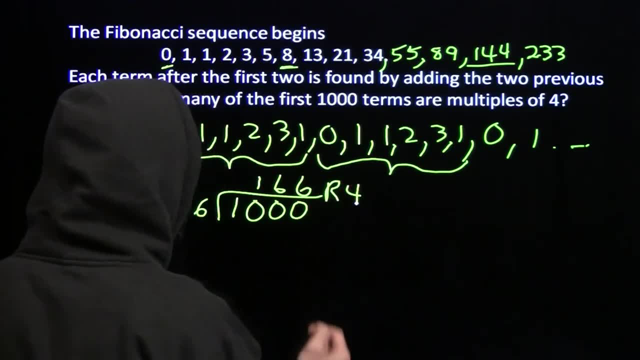 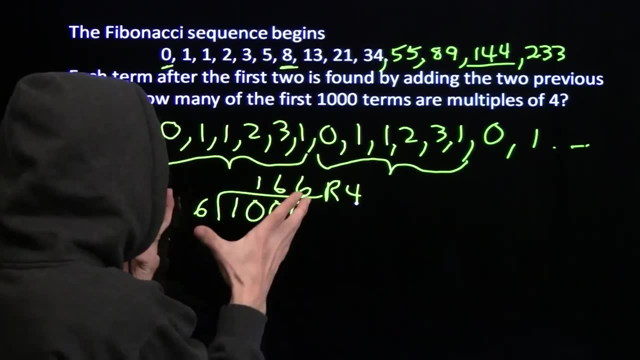 So if I take this thousand and I divide six into it, see, I'll get a one sixty six and I'm going to have a remainder of four. So that gives me- ooh, I've got to be careful here- I mean, it gives me 166 blocks of six. 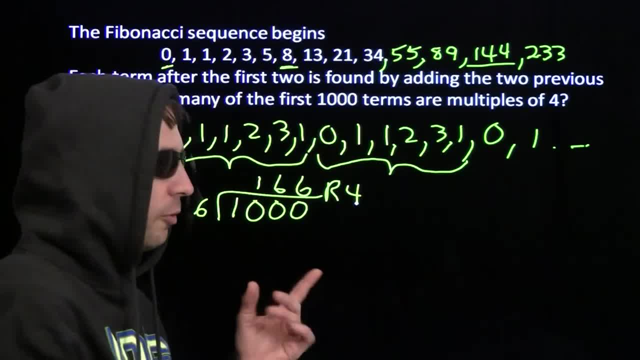 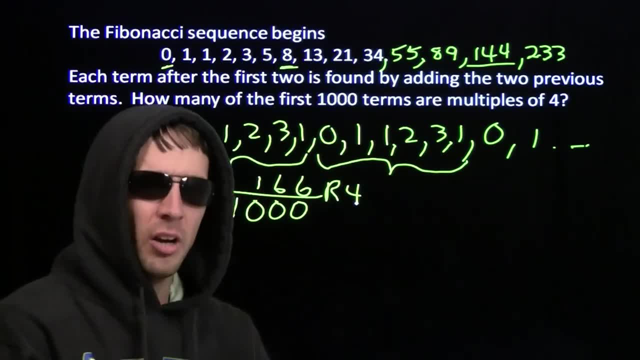 like this, and each one of those blocks has a single multiple of four, so I might write down 166, but I've got to be careful in these pattern problems and when you're counting things out like this, make sure you're not off by one. 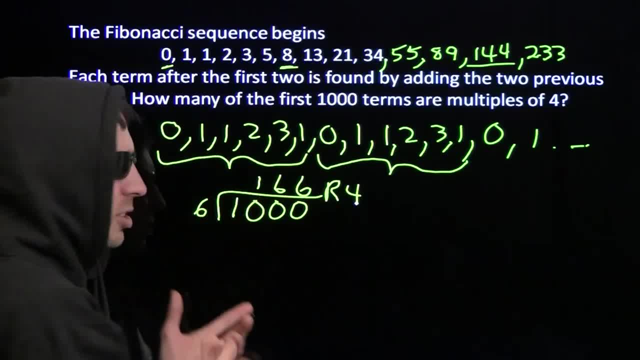 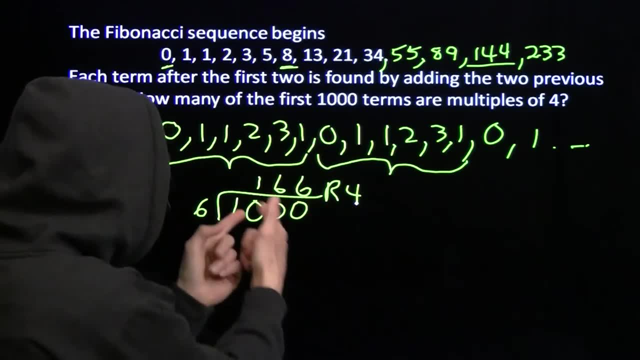 What's this remainder four all about? When I divide six into a thousand, I get 166.. That tells me I've got 166 of these blocks, but I do have four terms left over. So I go through 166 of these blocks. that gives me 166 multiples of four. but then I 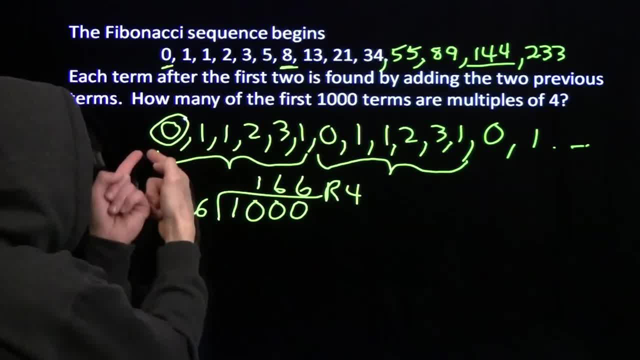 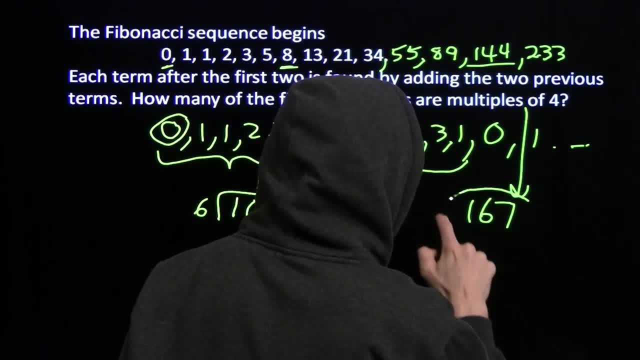 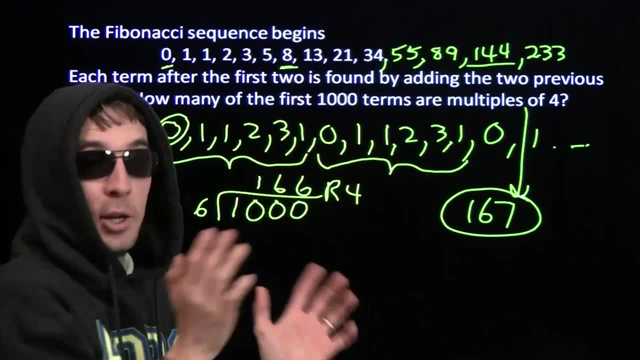 go four more terms And in those four more terms will be one more multiple of four. So that gives me a total of 167 multiples of four. Alright, so moral of the story here is find a pattern and a good way to find a pattern.